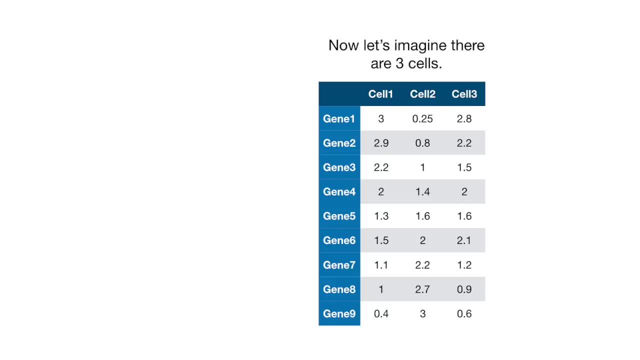 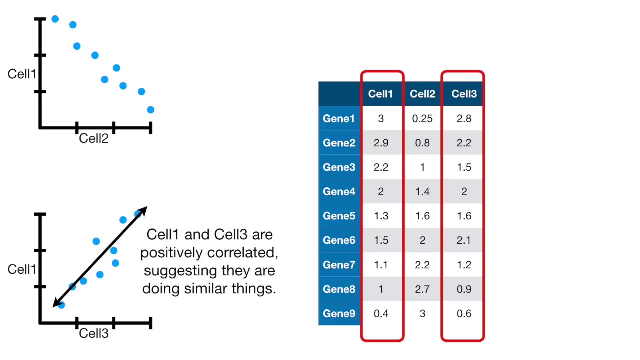 genes. Now let's imagine there are three cells. We've already seen how we can plot the first two cells to see how closely they are related. Now we can also compare cell 1 to cell 3.. Cell 1 and cell 3 are positively correlated, suggesting they are doing similar things. 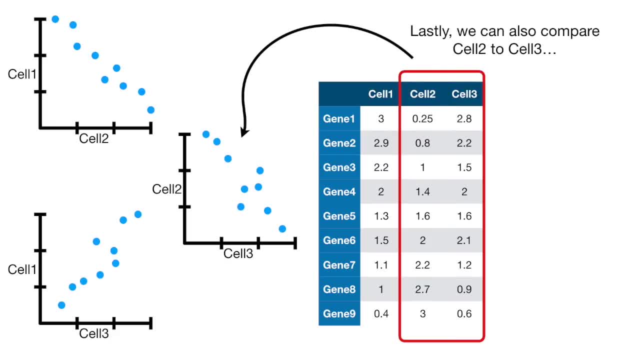 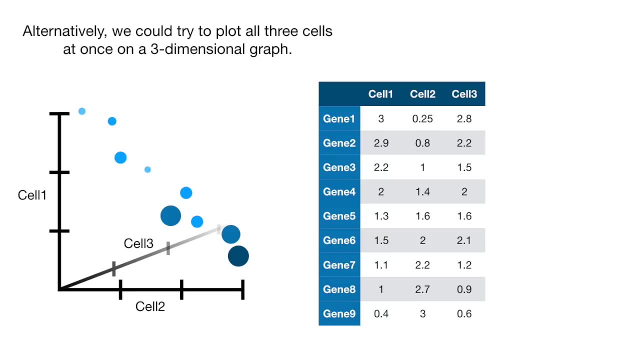 Lastly, we can also compare cell 2 to cell 3.. The negative correlation suggests that cell 2 is doing something different from cell 3.. Alternatively, we could try to plot all three cells at once on a three-dimensional graph. Cell 1 could be the vertical axis, cell 2 could be the horizontal axis and cell 3 could 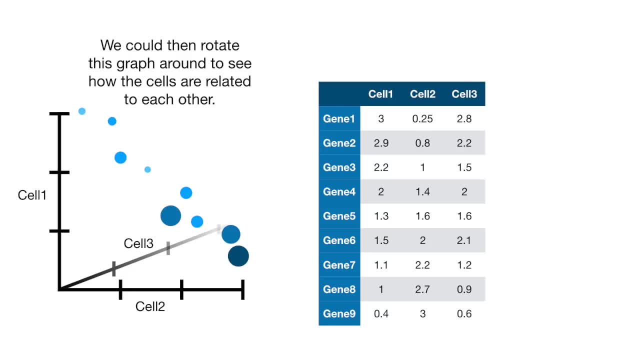 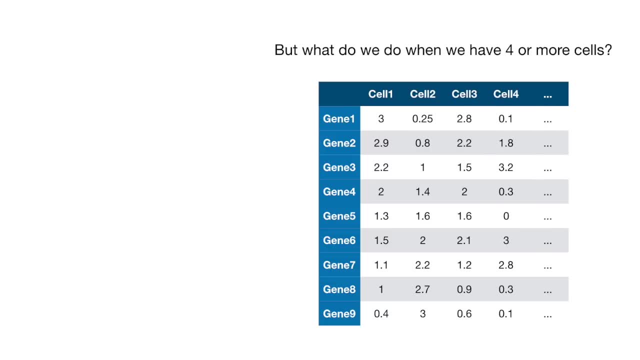 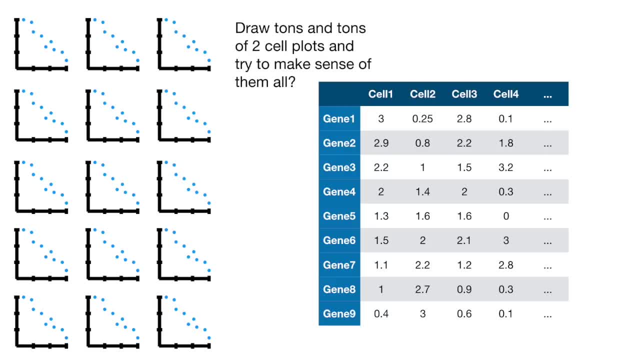 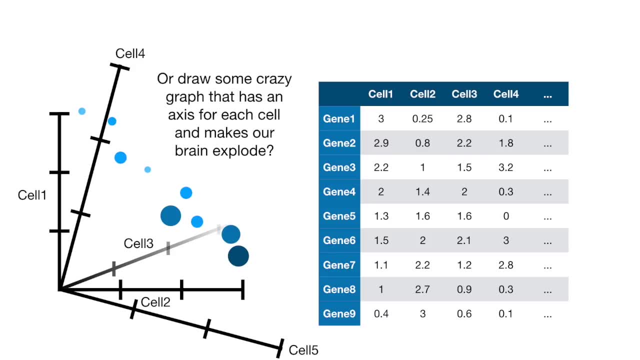 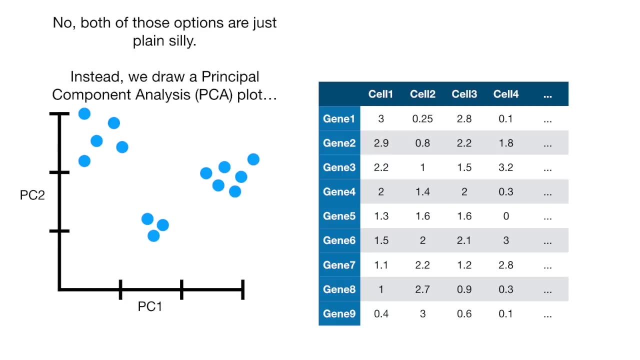 Draw a graph. Do we draw tons and tons of two-cell plots and try to make sense of them all? Or draw some crazy graph that has an axis for each cell and makes our brain explode? No, Both of those options are just plain silly. 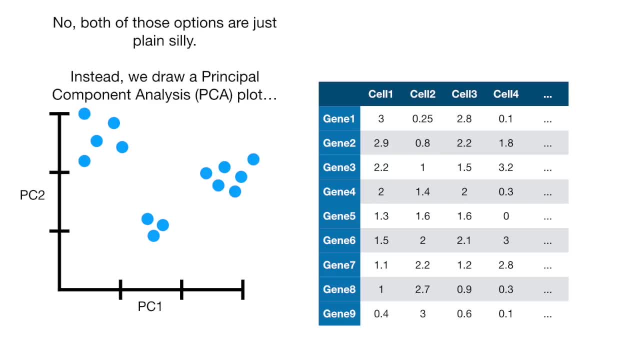 Instead, we draw a principal component analysis, or PCA plot. A PCA plot converts the correlations among the cells into a 2D graph. Cells that are highly correlated cluster together. This cluster of cells are highly correlated with each other, So are these. 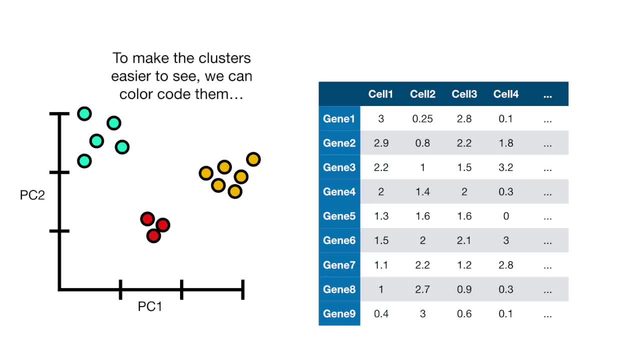 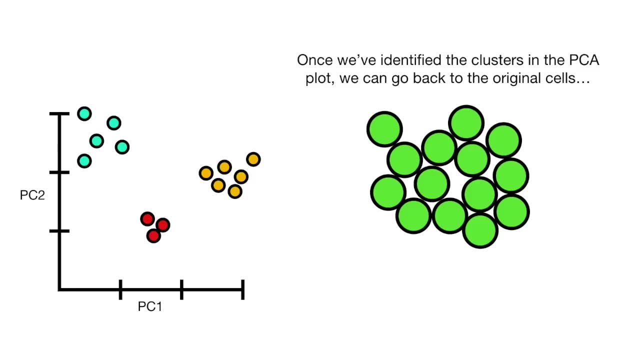 And so are these. To make the clusters easier to see, we can color code them. Once we've identified the clusters in the PCA plot, we can go back to the original cells and see that they represent three different types of cells Doing three different types of things with their genes.